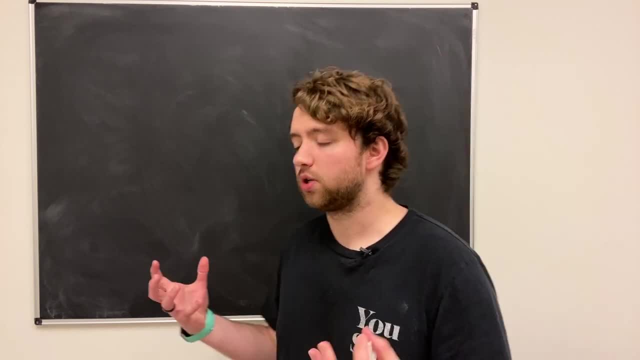 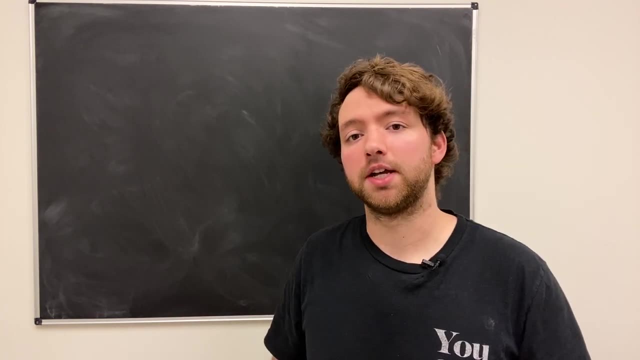 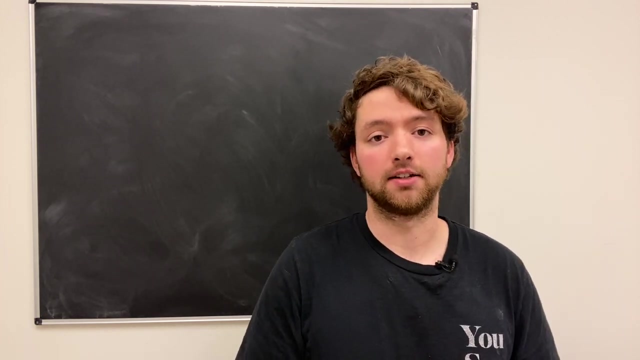 variables. No one wants to do that, So you can basically group a bunch of data together. Consider these like buckets, that you can put things in. A common term, you might hear, is a collection, a collection of data. An array is an example of a collection, and so is a linked list Array. 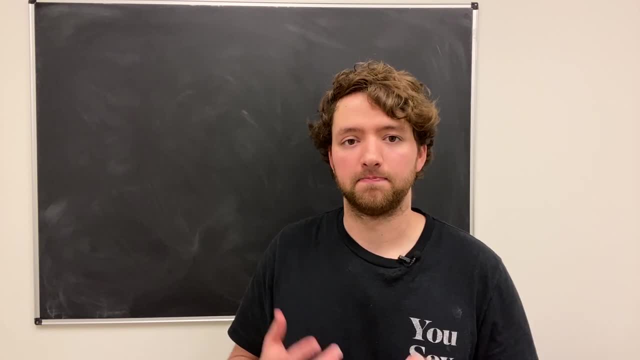 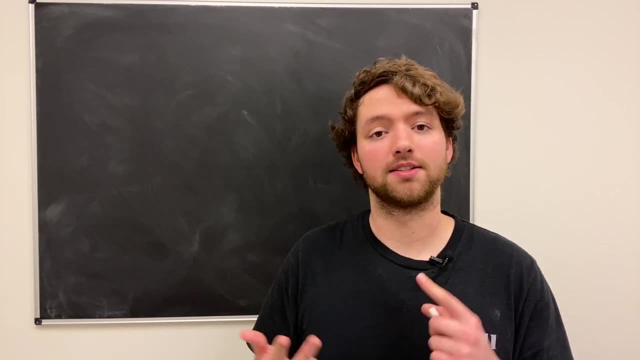 I would actually say there's two main types of arrays: There's a static array and there is a dynamic array. And there's a static array and there's a dynamic array And there's a static. so we actually have three things. we're going to be talking about static arrays. 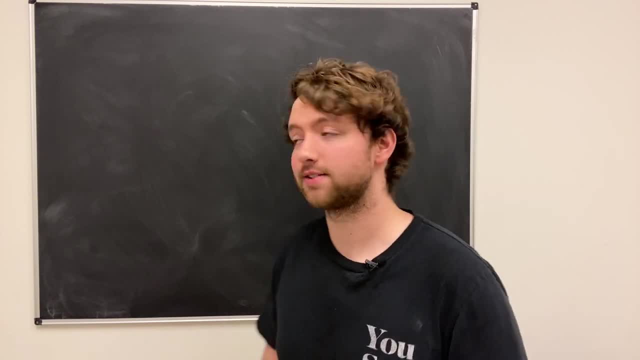 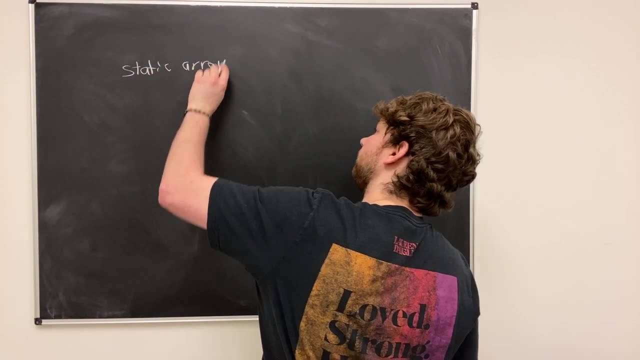 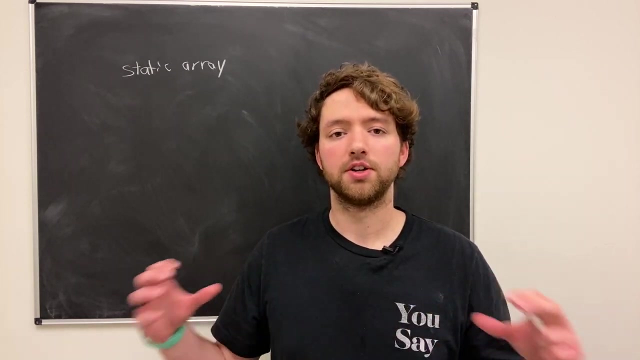 dynamic arrays and linked lists, and hopefully by the end of this you'll know which one to use. so let's talk about the first one here: static array. the thing about a static array is that in memory, in your computer's RAM, all of this stuff is stored sequentially together. so I mean, I'm not gonna draw a beautiful 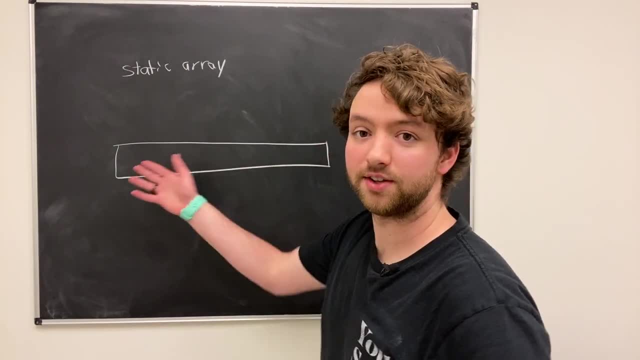 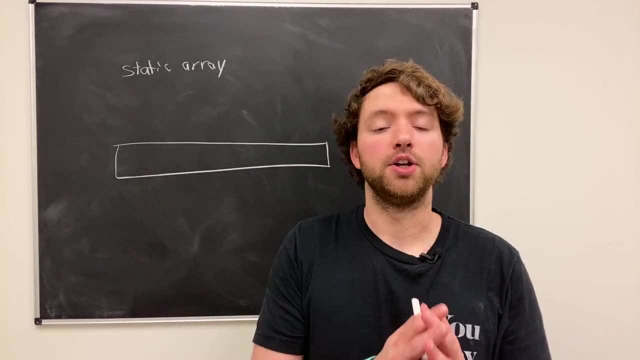 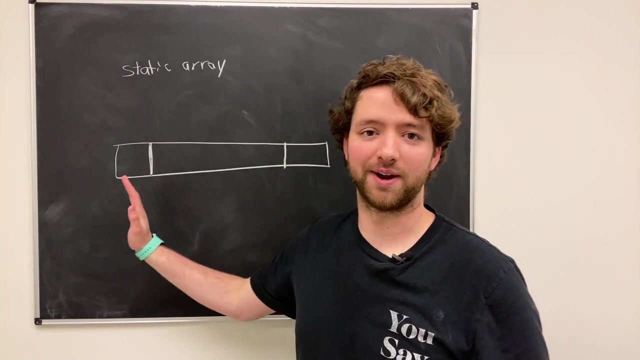 picture, but we'll try my best here. alright, so let's say this is your computer RAM and you can store an integer here, or you can store a string, whatever you need to do. but you actually want to store multiple pieces of information. so you block off some section of your RAM and in here you 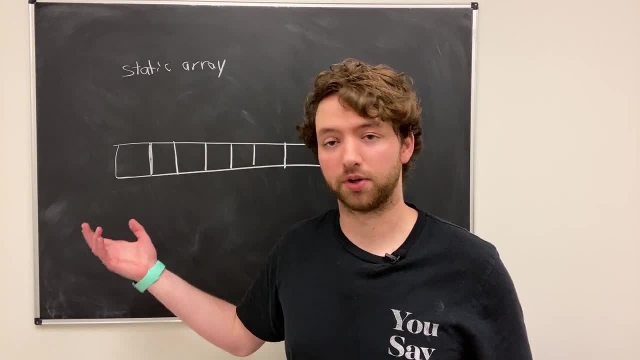 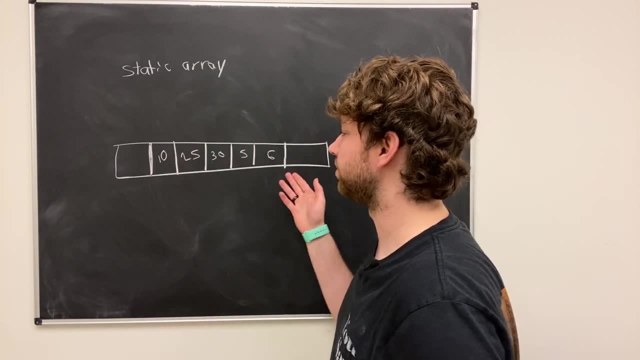 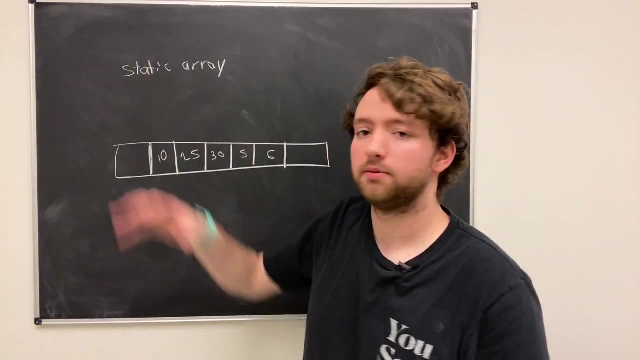 split it up into different spots where you can store data, so you can put numerous numbers in here and it's all sequential inside of memory. when you're dealing with a static array, the keyword static here means that it doesn't change once you determine that size it's going. 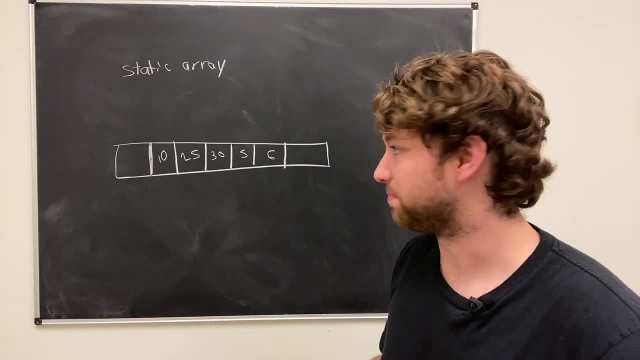 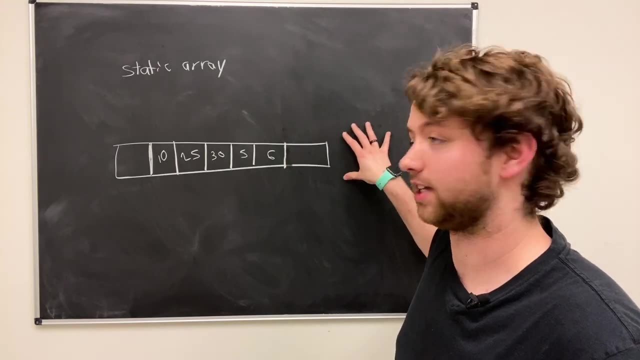 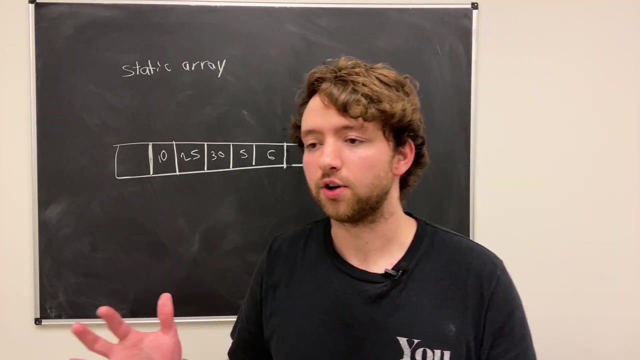 to forever be that size. a common issue that people have is they will add data at the end of it beyond the max, or they'll try to access data that's not actually there and that'll throw an exception or make your computer explode or make you lose your job or all of the above. so if you 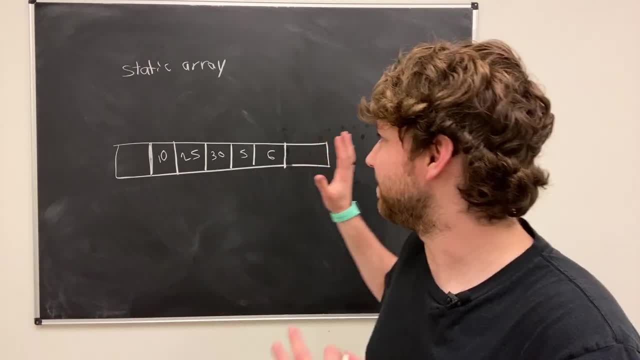 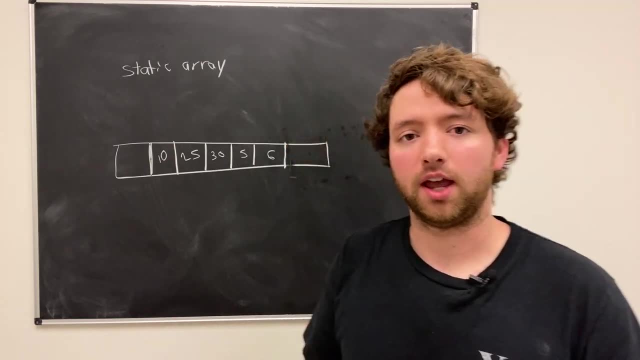 want to be like a failure, do that. but if you want to be a good developer, don't do that. so you always have to keep track of that list. so if you're working with a programming language like C, first off. I'm sorry, I feel bad for you, but you're. 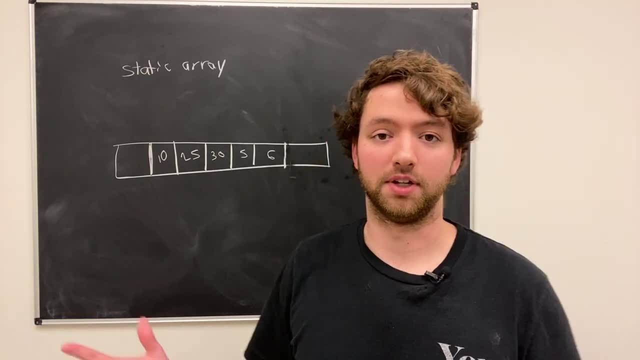 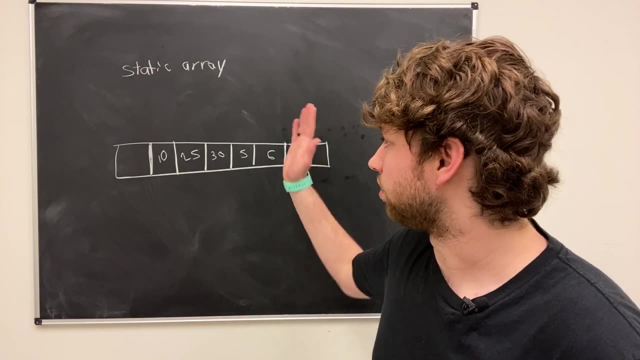 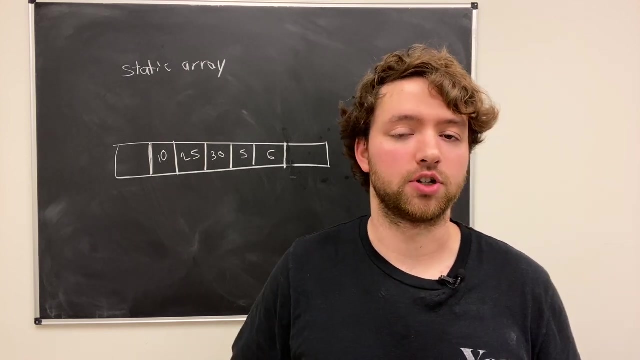 probably gonna have to keep track of the length of your list. so you often have another variable- you're passing around the functions- which is basically your array length. that way you don't go outside of the bounds. fortunately, with some of the other programming languages you're going to have some function to 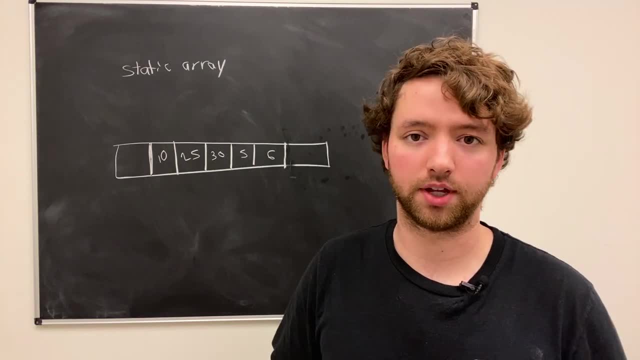 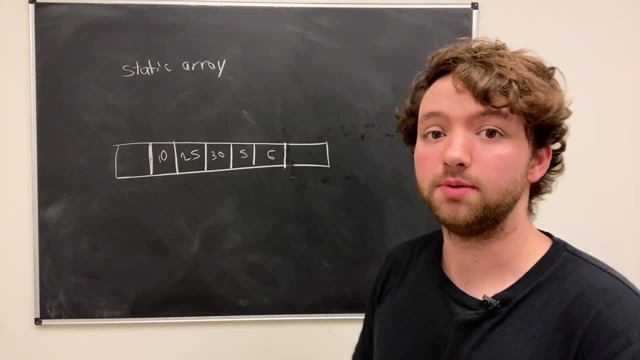 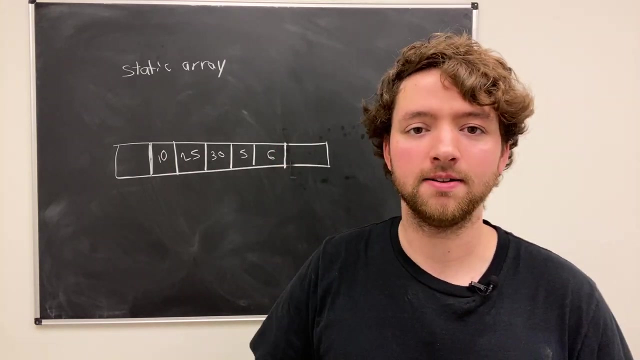 calculate the length, and it basically maintains that knowledge with it, which makes our lives a whole lot easier. but with a static array you have to keep track of that yourself and you're limited to that size. so if you think you're only going to need five spots and then you later find out you need ten, 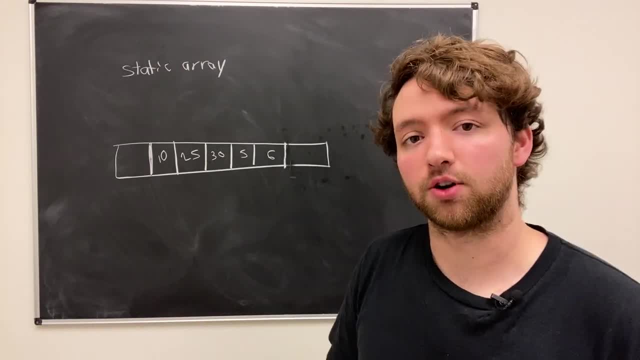 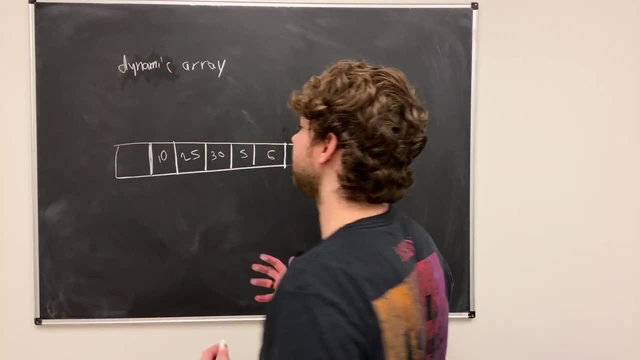 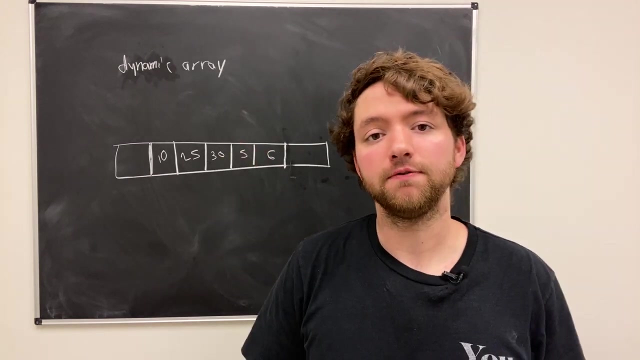 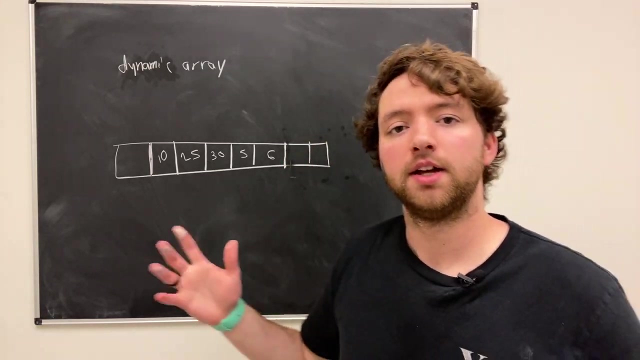 you're doomed. so this is where a DUNGEONMATCHCOM dynamic array comes in. now, a dynamic array, you can use it just like a normal array. it works the same way in memory. the difference here is that if you say, hey, I want to add an element, and you go outside of the bounds of that array, it's. 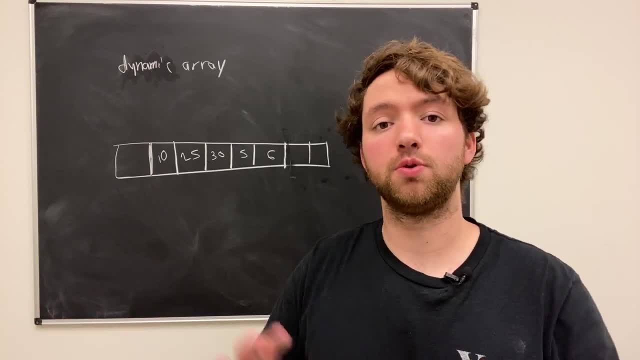 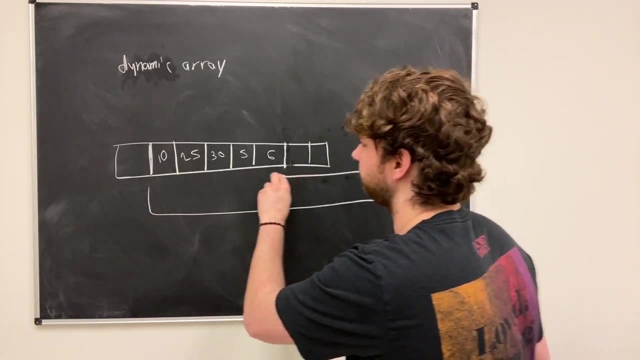 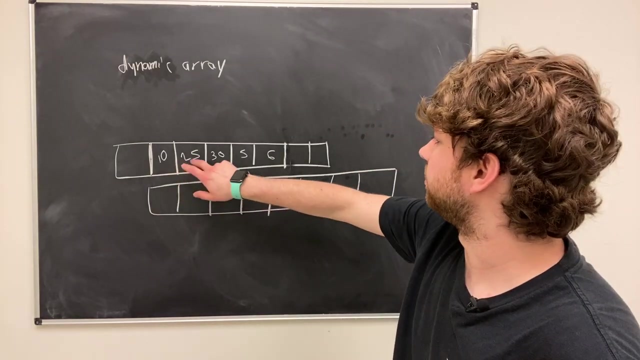 going to catch you and it might just be behind the scenes, you won't even know, but it will actually create a new array. so it's going to create a new array for you in memory and it'll probably like double the size. so we have one, two, three, four, five, five, six, seven, eight. you probably end up. 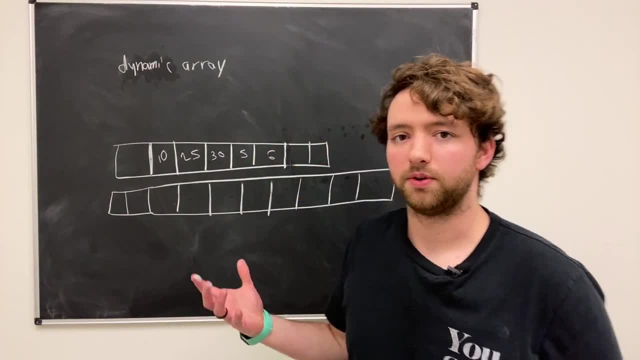 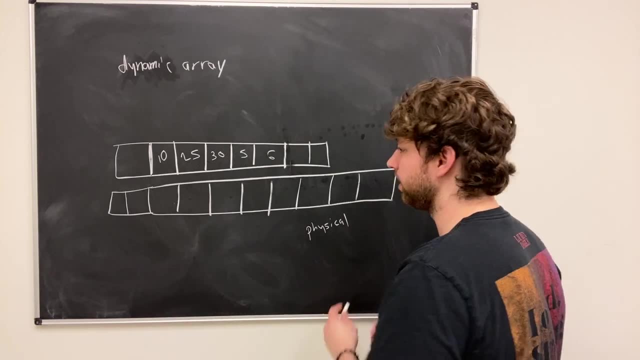 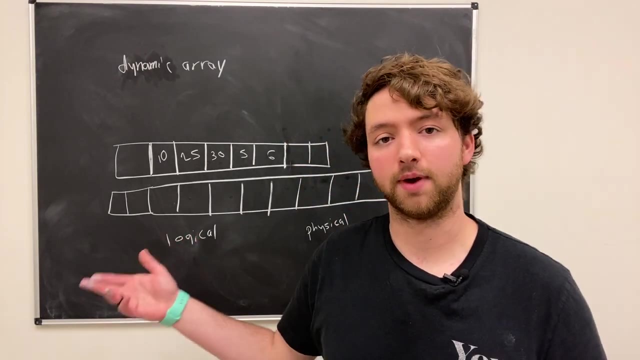 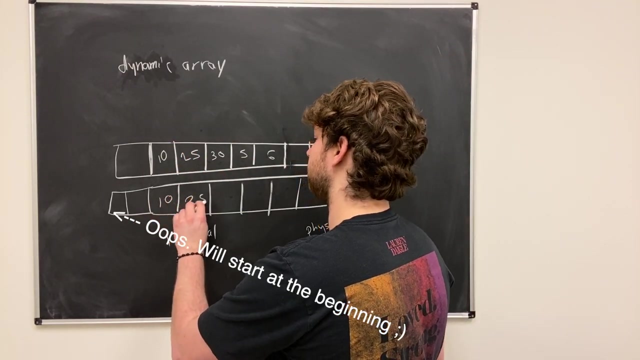 having ten spots. so in this situation you have pretty much a physical length- how much room it takes up in memory- and you also have a logical length, which is how many elements you have in it. so behind the scenes, this will actually be copied over to this larger array. so you'll have ten, twenty five. 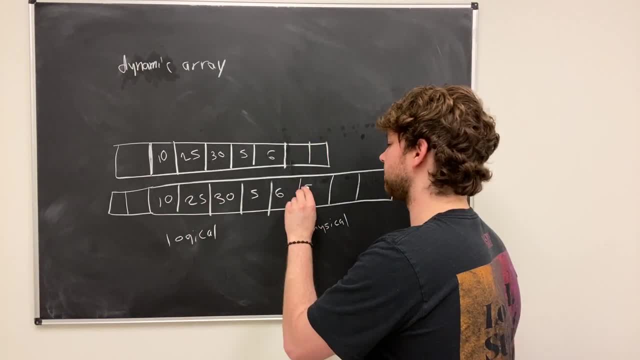 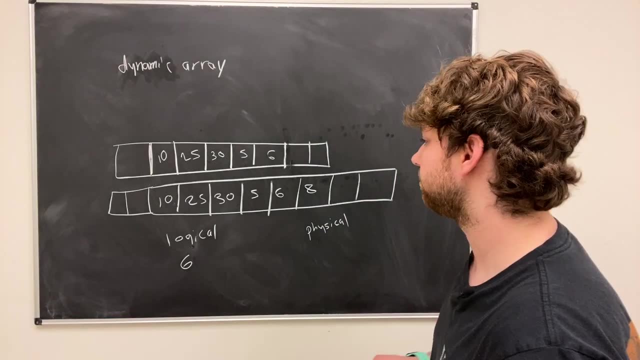 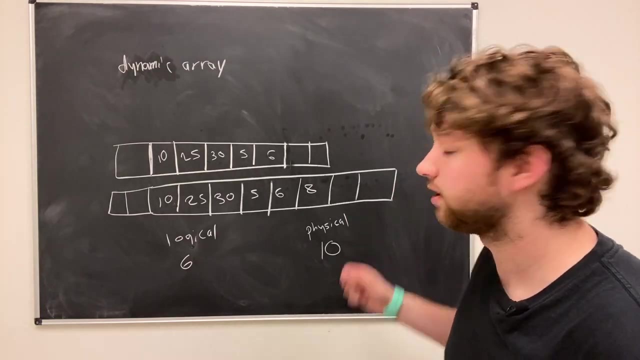 thirty five, six, and let's say you added the element eight doesn't really matter. so the logical length here is going to be six. there's six elements. the physical length here is going to be ten. whenever this logical length is increased beyond the physical length, the physical length will increase. 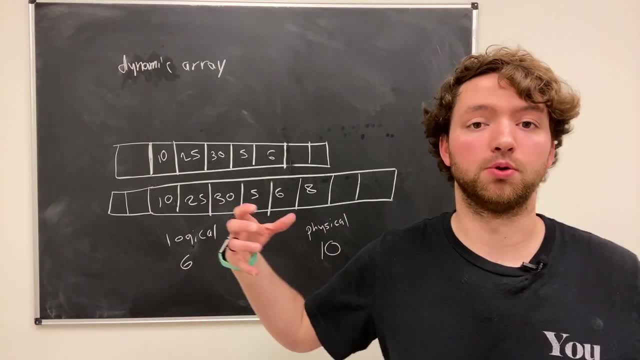 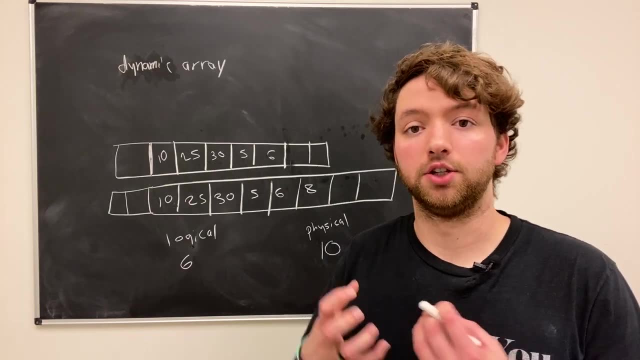 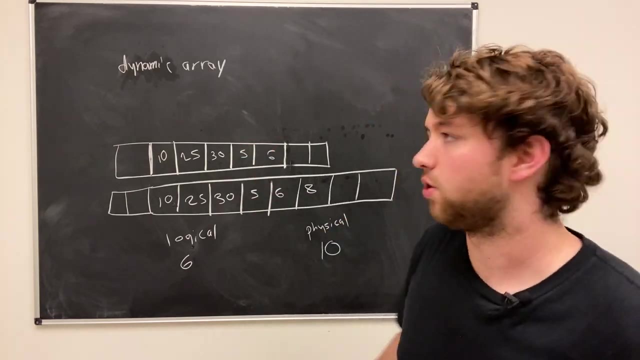 likely doubling. so if you go above ten, it'll likely double to twenty. so that is how a dynamic array works and from the developers perspective, the the user of this dynamic array. we do not have to worry a whole lot about this process, it just works. so you probably have some variable and we'll just call it. I don't. 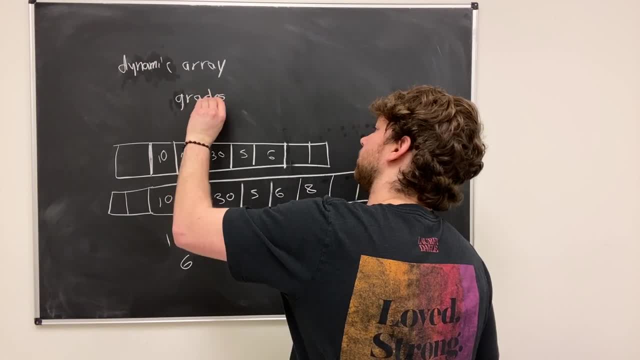 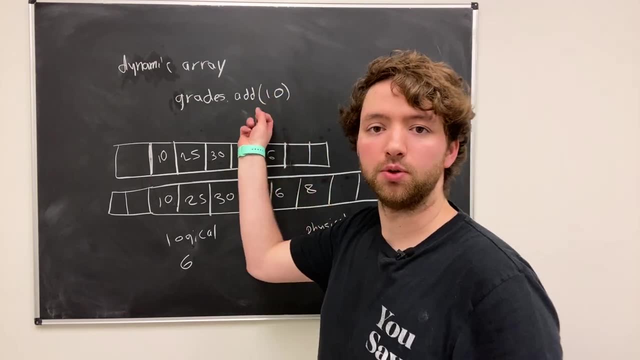 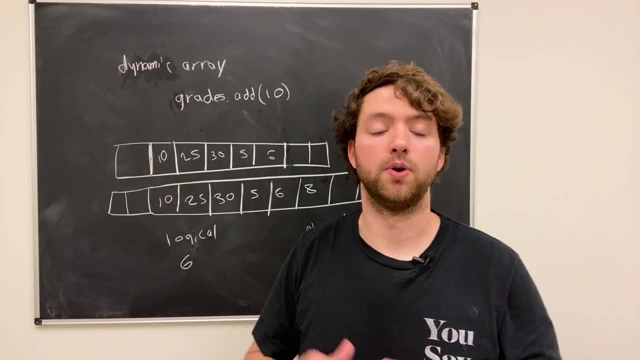 know something like grades, and there'll be a method such as add or append and you can pass some data in here and you can just keep doing this. if the logical surpasses the physical, it'll automatically increase the memory size, so you don't ever have to worry about it. so that is the beauty of a dynamic array. 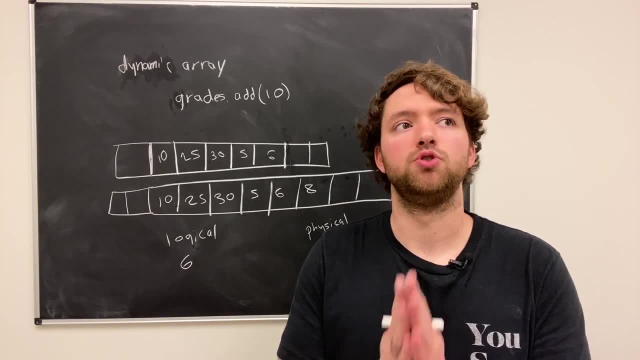 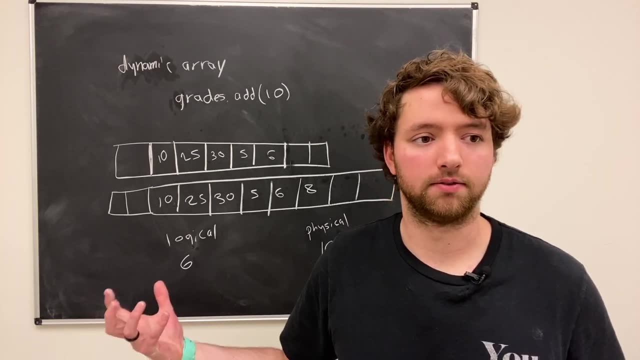 and whenever you can use a dynamic array over a static array, do it. unless you're a hundred percent positive, you're never going to need more than a certain number of elements. then you don't have to worry about it. so if you know ahead of time- meaning when you're coding, and you're coding and you're doing the other stuff- 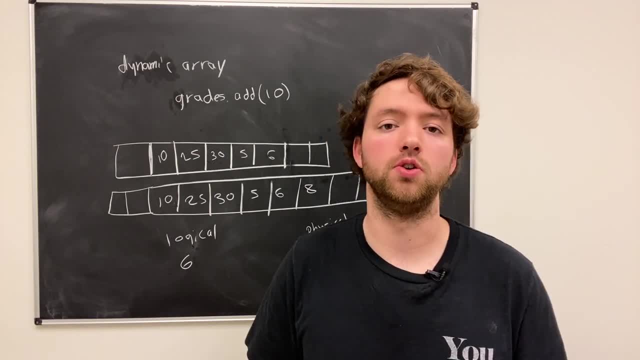 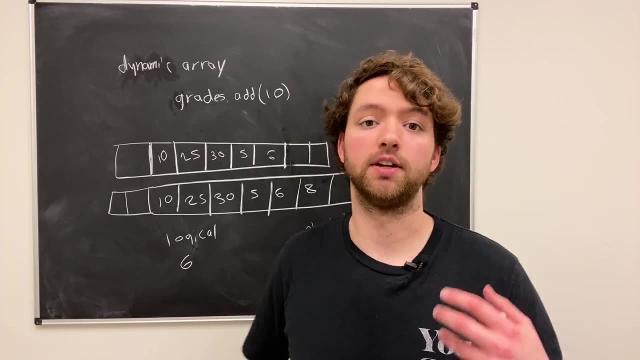 the application, how many spots you're going to need. you can use a static array. Static meaning you know it up front. If it can change, such as reading from a database, or reading from a file, or asking the user for input, well, you don't know how many values are going to be there. 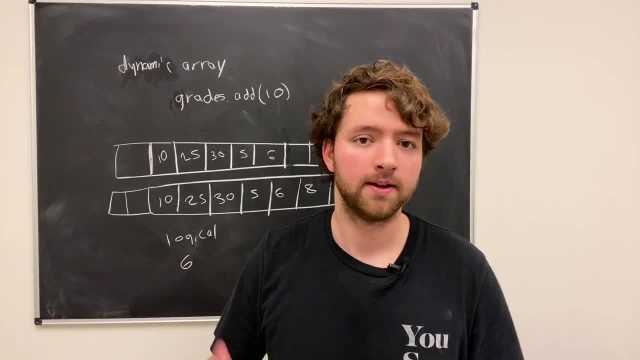 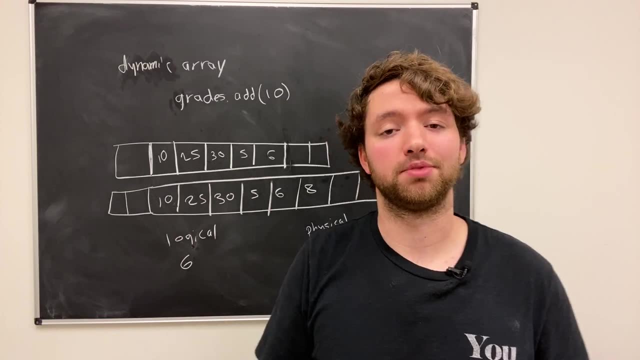 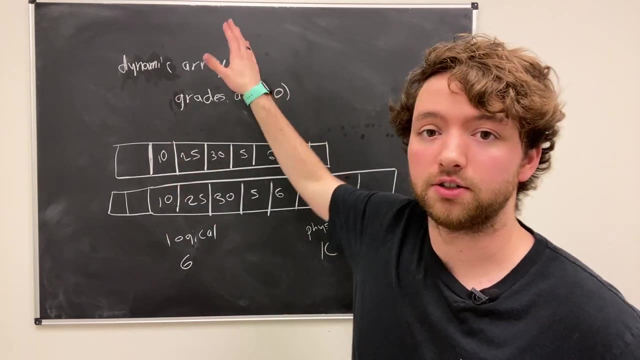 so in that situation you will want to use a dynamic array. You can probably build something like this in C, but there's not a real easy way to do it. by default In C++ they introduced the vector that makes everybody's lives a whole lot better. Inside of Java you got the array list. 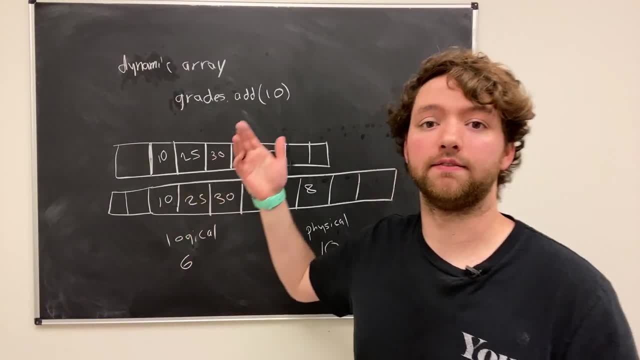 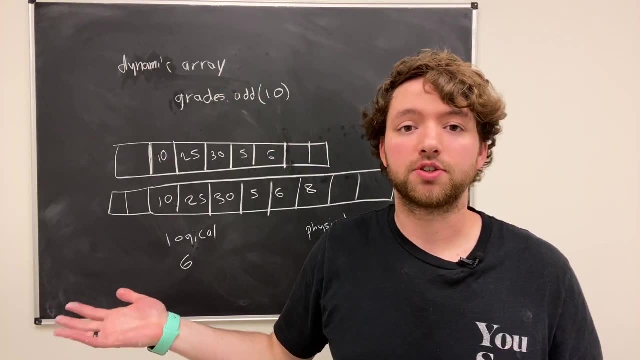 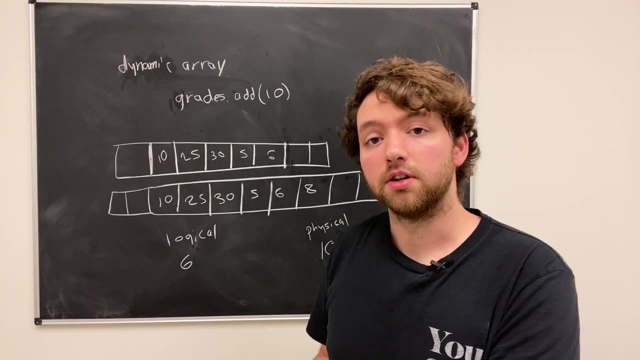 same with C sharp. In Python you have a list, so a list behind the scenes is a dynamic array, and that pretty much sums up most of what you're going to be using inside of modern programming languages. Now the other one that we want to talk about is 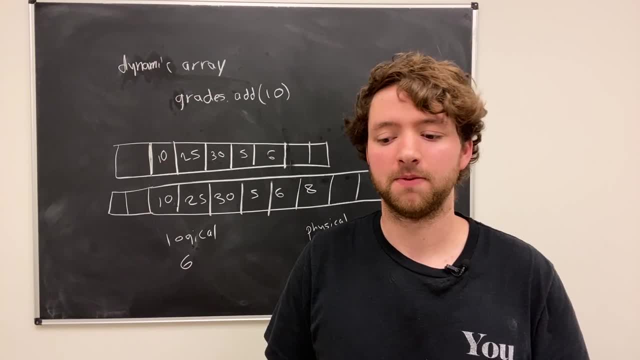 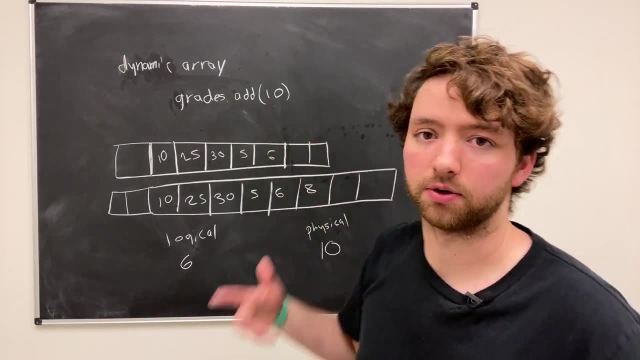 a linked list and this works a little bit differently. The actual interface for working with the linked list might be the same, you know. you still might be able to say dot add or dot append. you still might be able to get things by index. so you might be able to say: 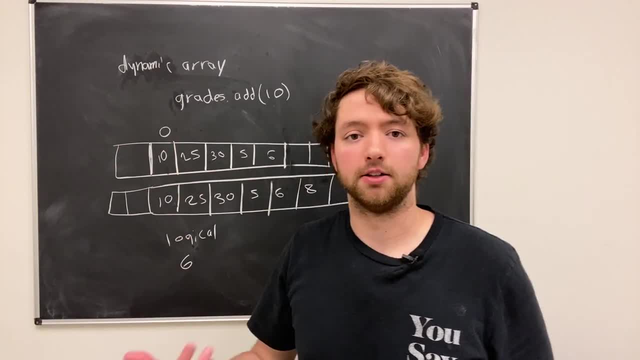 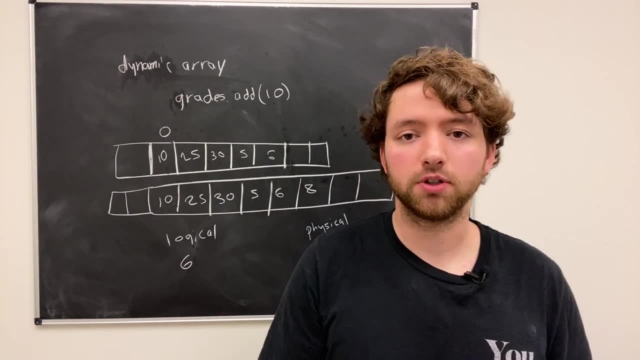 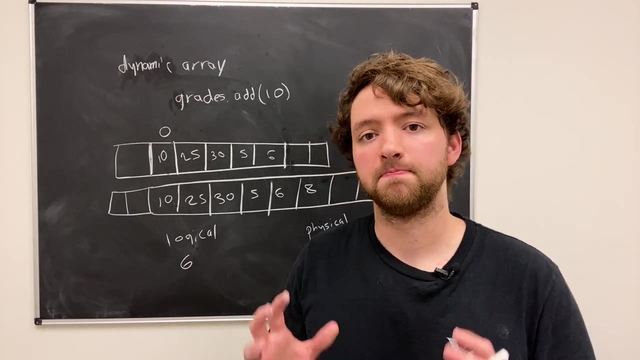 hey, grab the thing with the index zero and grab that element, But structurally and the performance is different. so it's structurally different and it performs differently. So let's talk about what a linked list might look like. do that? there's one more thing I want to show, and that is: in this situation we are storing the 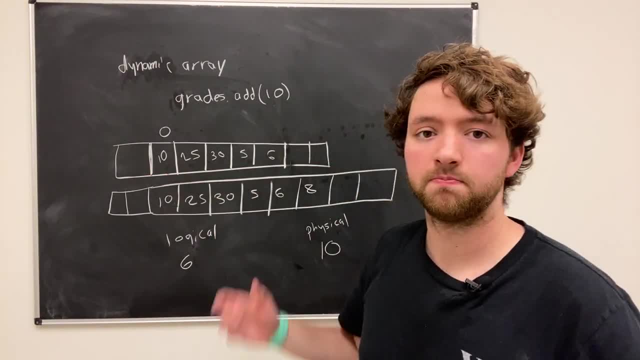 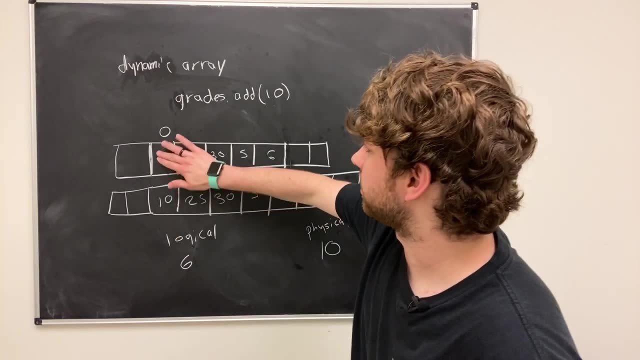 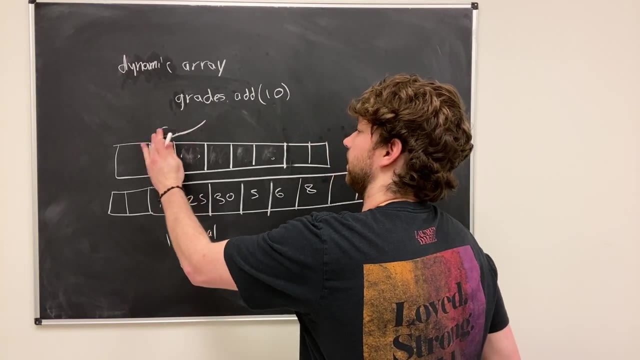 elements directly inside of these spots in memory. You could also have a situation where, instead of storing them directly, you're actually storing pointers. So in that situation it's no longer going to look like this, It'll look like this. So let me actually- here's a pointer to the value 10. 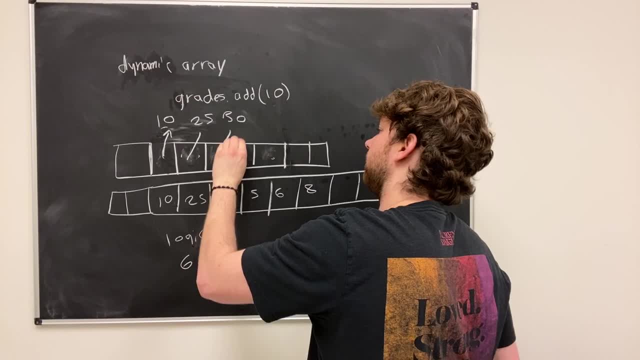 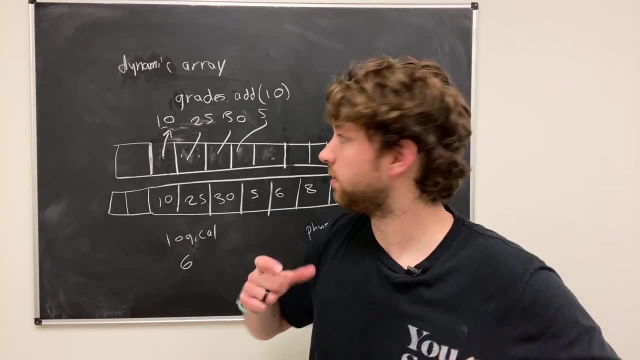 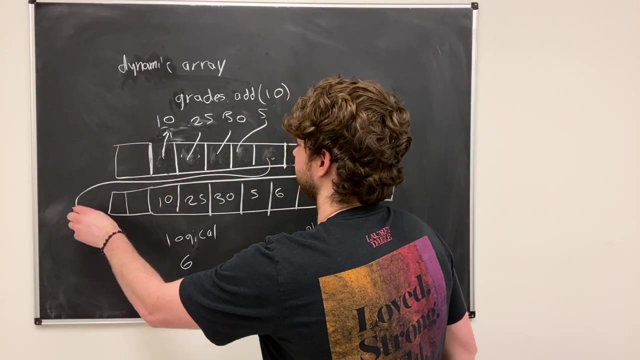 here's a pointer to the value 25- and in this situation the array itself is sequential in memory, but the data it points to can be anywhere in memory. So, for example, this one can be somewhere totally different, but you can still read through the data just the same way. The only difference is: 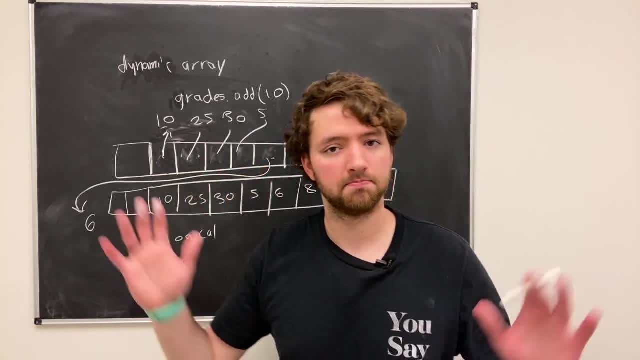 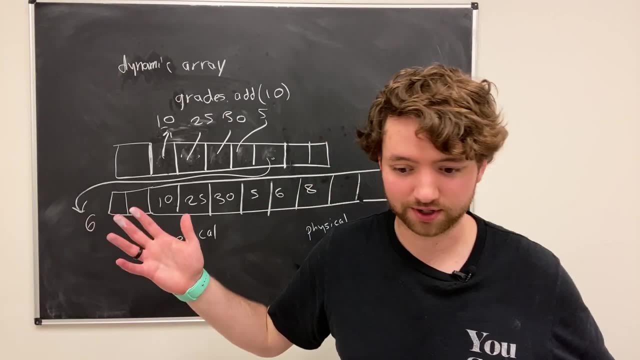 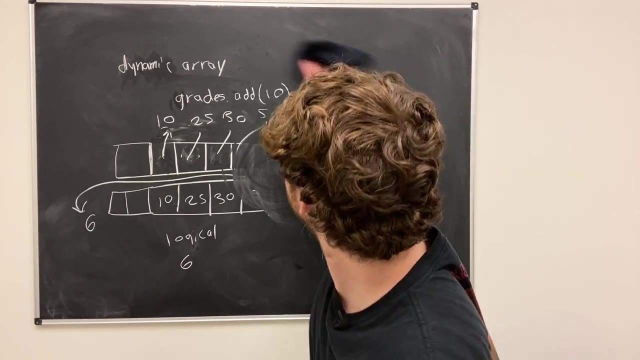 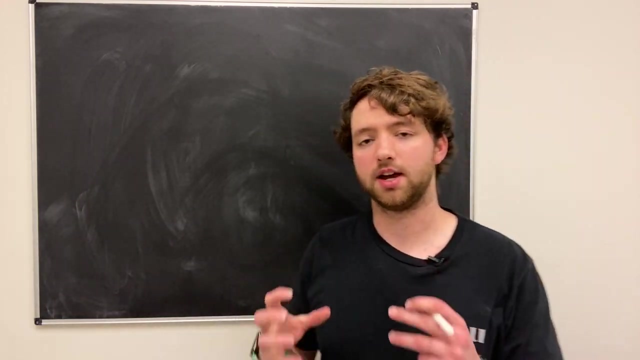 with this, you have just an additional pointer for each element, No big deal. So that's all I got for array. And now let's talk about linked lists, and of course I forgot my eraser. No problem guys, I got it's out here. So with a linked list, you're going to basically have a node, a thing to store the data. 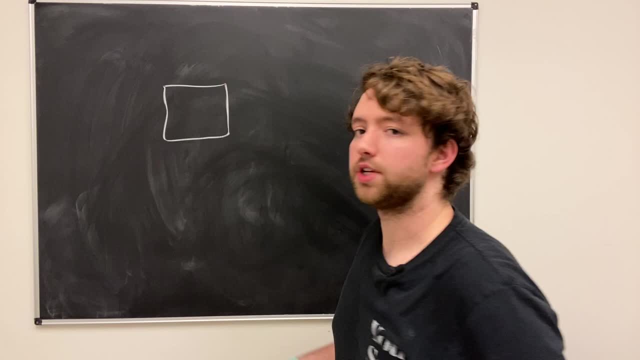 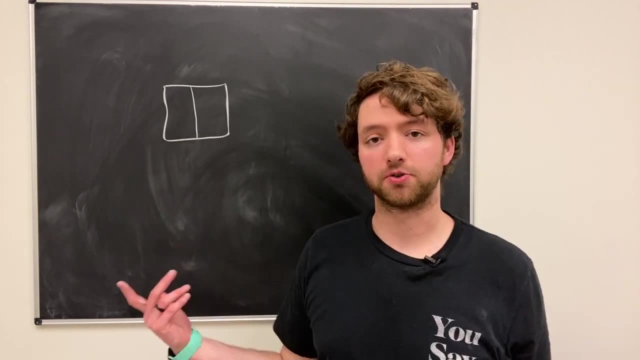 and when you do this, this node is going to have two pieces. So we'll split this. The first piece is going to be a node and the second piece is going to be a node. So we're going to have a node and the third piece is going to be what you're trying to store. So let's say we're trying to store 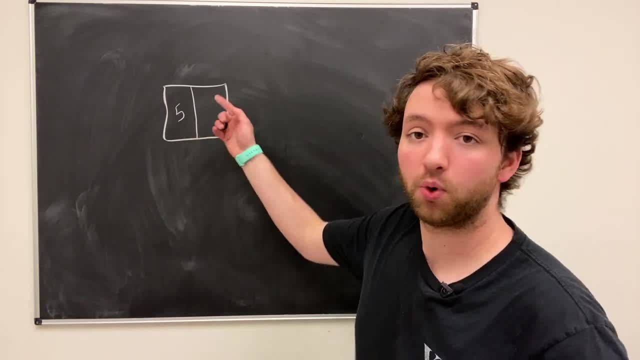 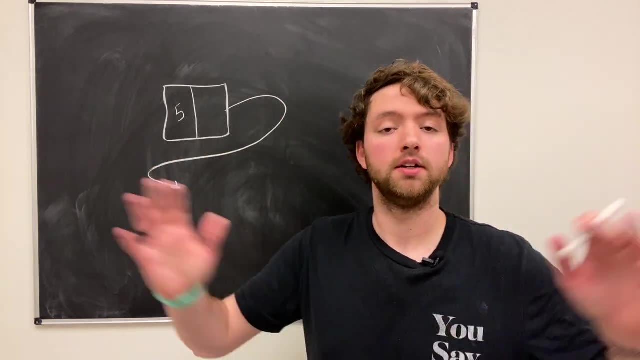 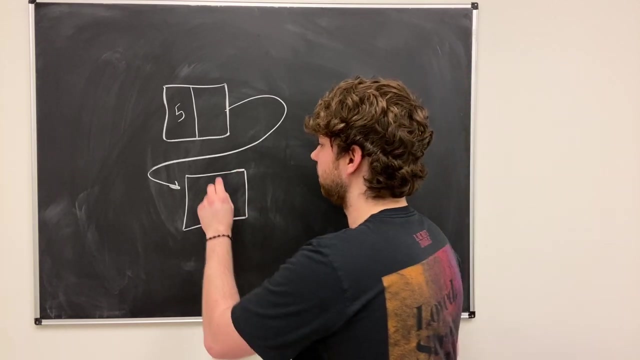 the number five. The next piece is a pointer and this will point somewhere in another spot in memory. So here's the magic here. it doesn't have to be sequential. It can point anywhere in memory and it's going to point to another node. Inside of this node you're going to have another piece. 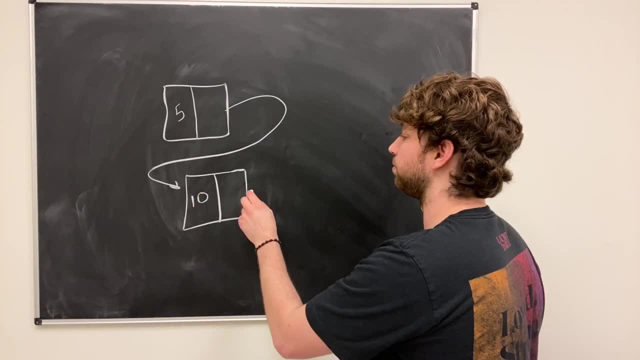 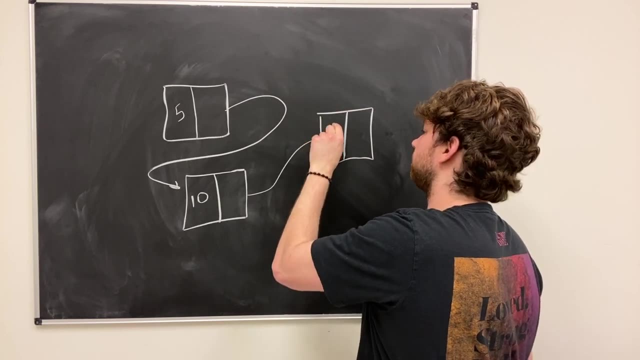 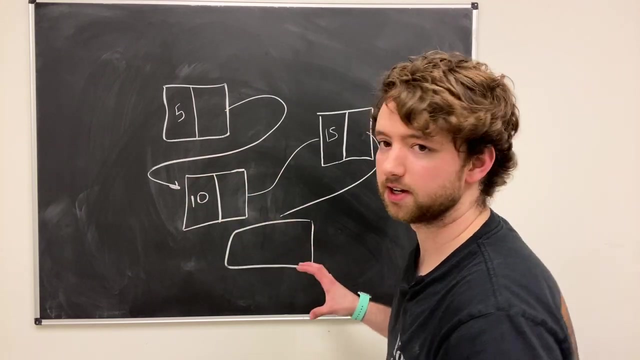 of data, We'll say 10, and then we got another pointer which can point somewhere else in memory, And we just keep repeating this process. Let's say we have the value 15 and we point somewhere else. I'm drawing it in this weird design just to show you guys that the location doesn't matter. 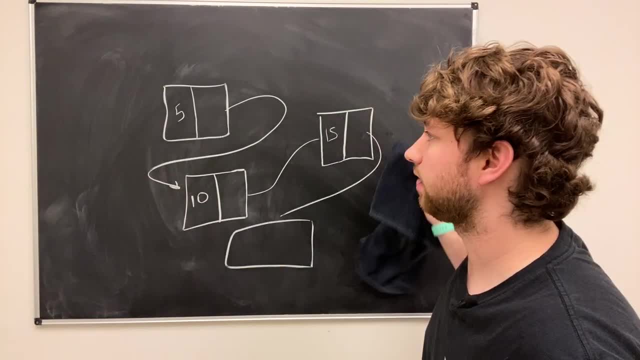 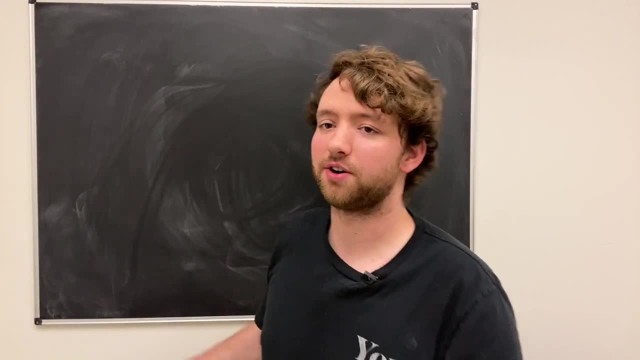 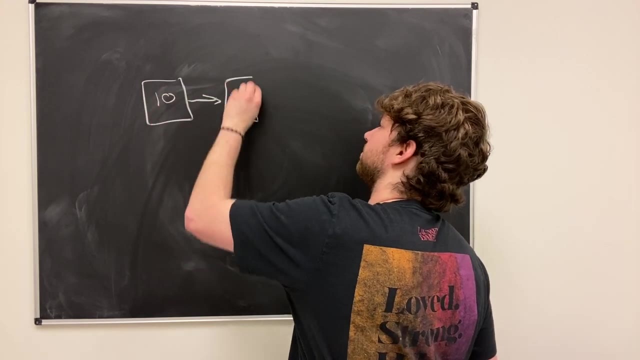 inside of memory. However, for sanity's sake, people often think of a linked list as a straight line. So we could draw this data out to show how it's represented like. so We have 10. That points to some other value. 15. That points to some other value. 3. Doesn't really matter. 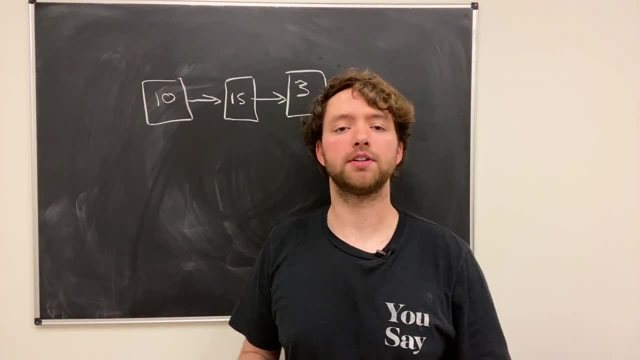 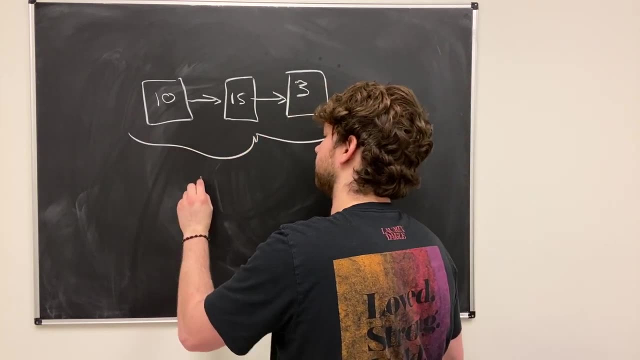 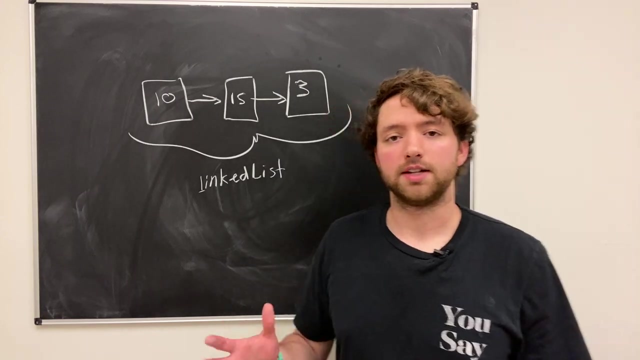 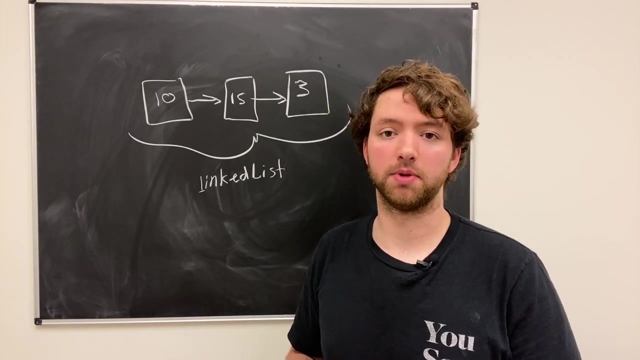 So you have these nodes and they'll all be connected and oftentimes you'll have some larger structure to contain it all. So you could say: this is your linked list. Now, linked lists are not as popular as dynamic arrays Because they have some serious downsides in terms of performance. 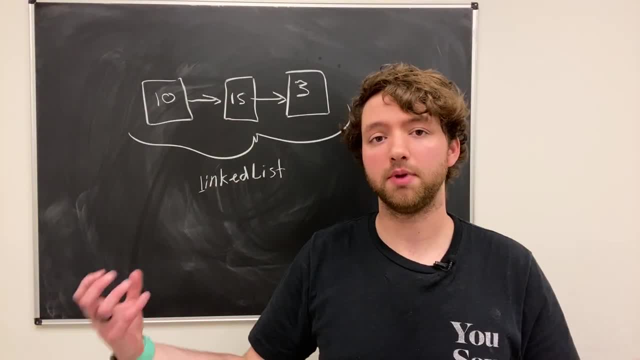 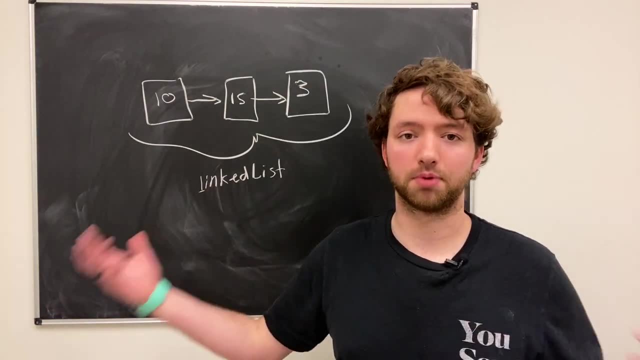 The obvious benefit is that it doesn't have to be sequential in memory, so it can point anywhere. And if you're always going to be going one element after the other, then a linked list is perfectly fine, Because you can go from this element to this element, to this element. 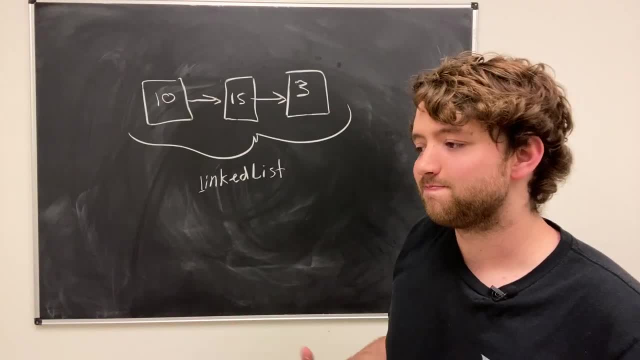 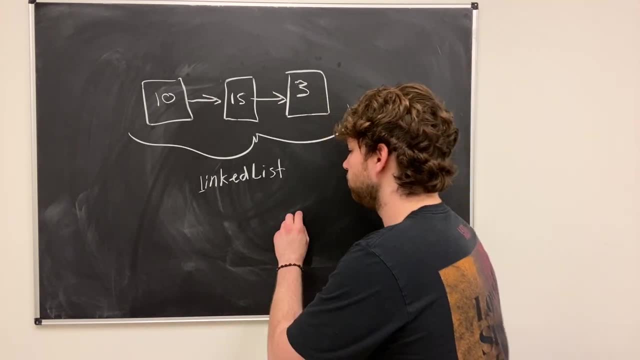 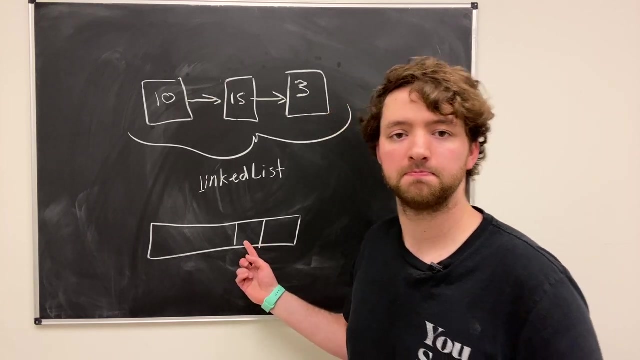 and keep going down the chain. However, grabbing any element by an index is not so easy, So you have kind of grown a bit from there. When starting with an array, you know that starting position. So if you wanted to grab this element here, all you got to do is find out the size of the individual boxes. 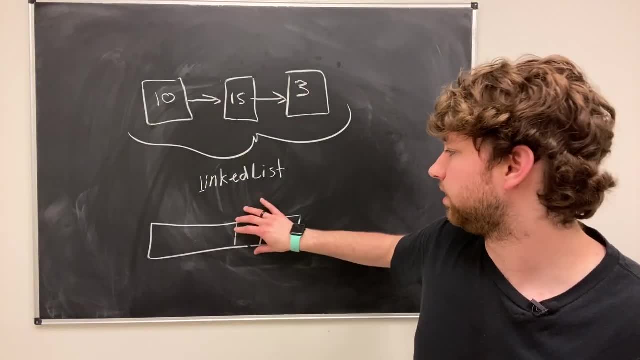 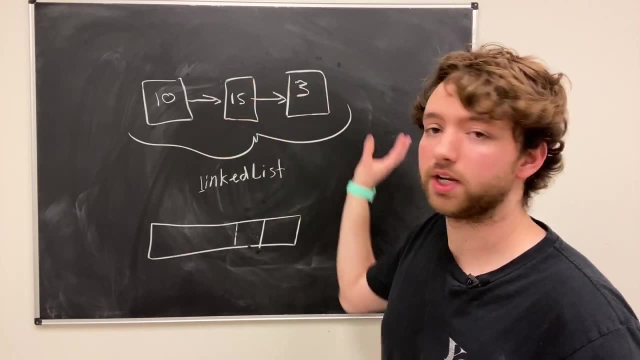 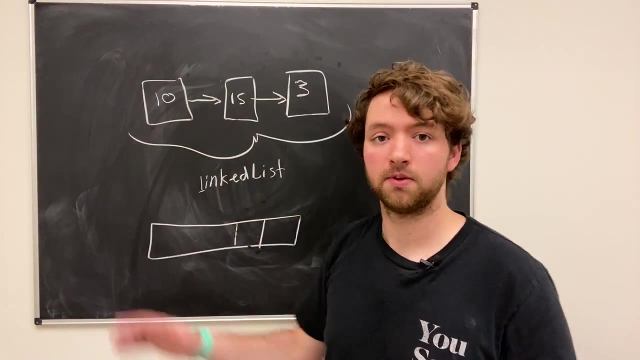 multiply it by the index you are trying to grab and you'll get the element or something like that. With a linked list it works a little bit different Because these can point anywhere, Anywhere in memory. We cannot just grab it and be done, So we actually have to start at the beginning. 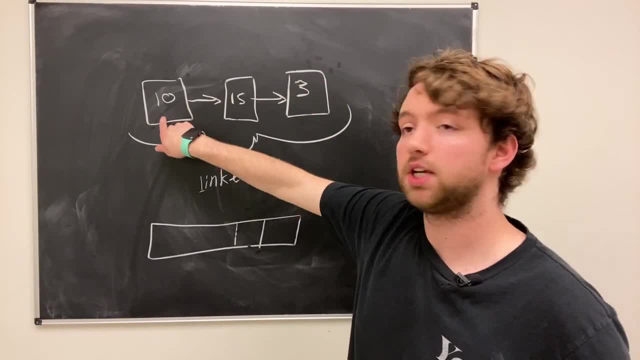 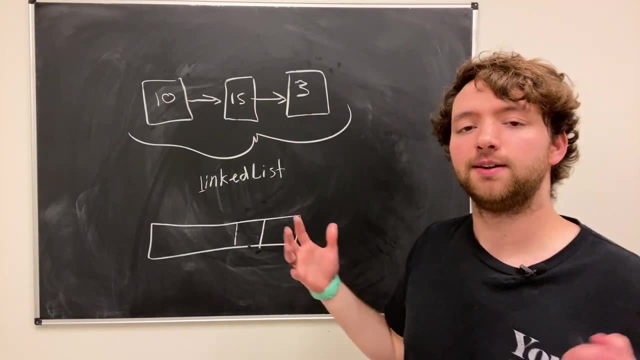 So if we're trying to get the third element here, we start at the beginning, go to the next position and then go to the next position And then we grab that element. Obvious downside here is that if you have a really, really large linked list, 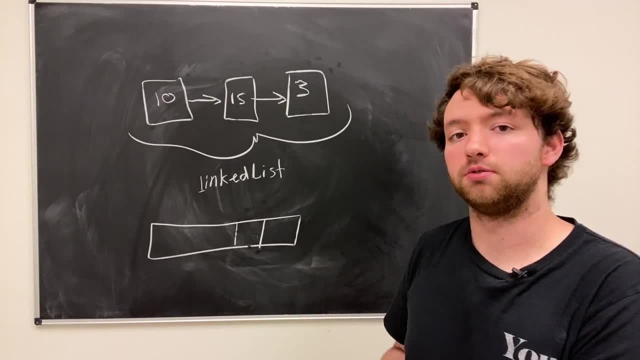 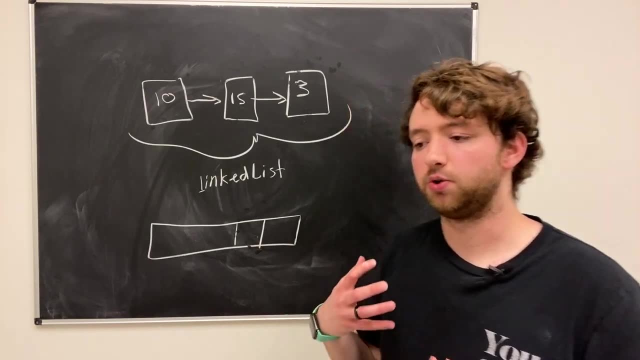 you're going to have to start at the beginning every single time you want to get a particular element. When you are working with a linked list, you can do the same kinds of operations. you can add elements in the middle, you can delete elements- Just the way you do it. 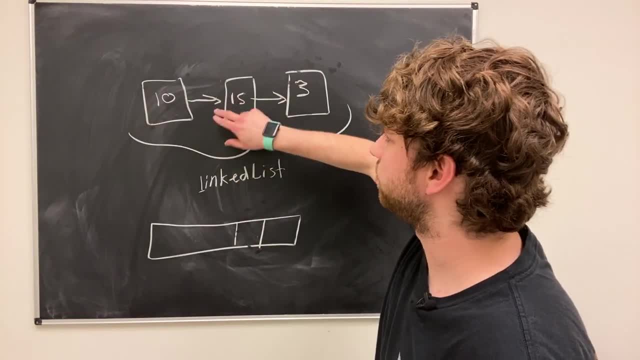 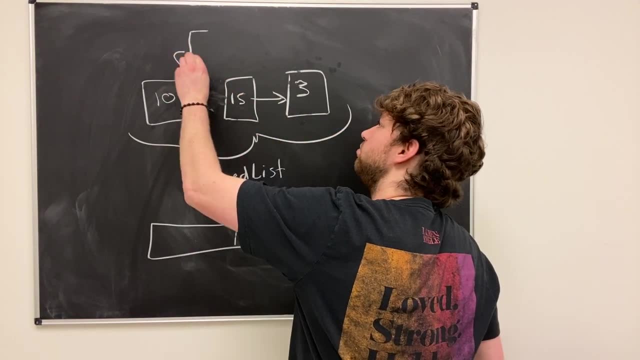 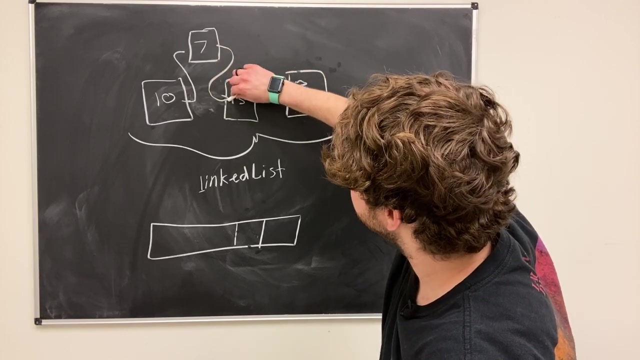 is a little bit different. So, as an example, if you wanted to add an element right here, all you would do is change this pointer to point to a new box, Let's say the value of seven, And then this box would point to this one here. So that is how a link list would work. Same thing. 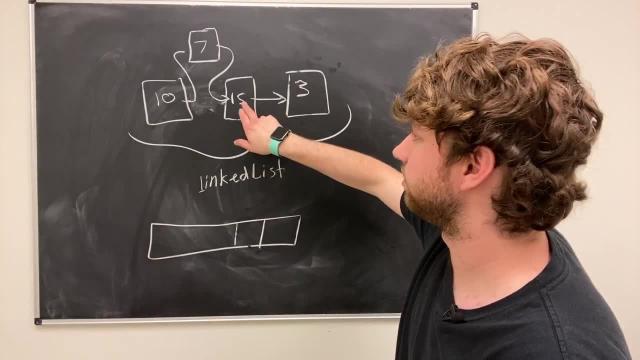 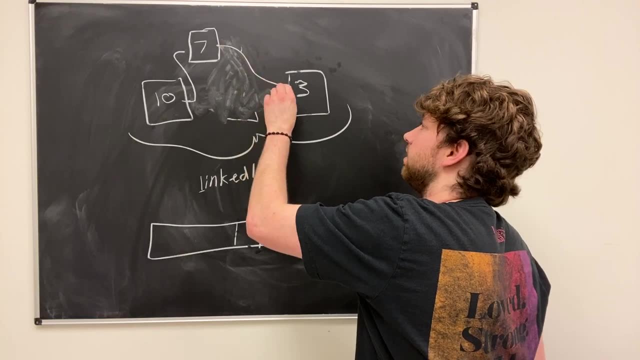 if you wanted to delete a node- Let's say you want to delete the link- you can delete the link this 15. all you got to do is grab the the node before it and make it skip it to go to the next node. It doesn't even matter if this one's still in memory. It's irrelevant because we don't have. 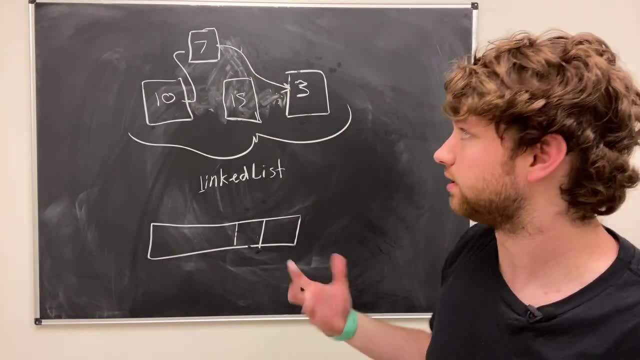 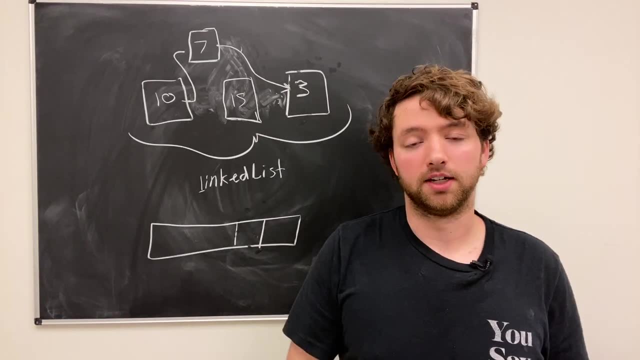 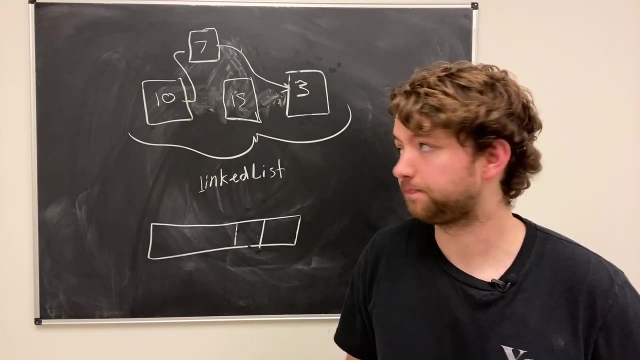 a pointer to it. So in our mind it's essentially not there, and garbage collection will get rid of it. So that is how a linked list works. So which one do you use? More than likely, most of the time, you're going to want to use a dynamic array, You will occasionally run into linked lists. 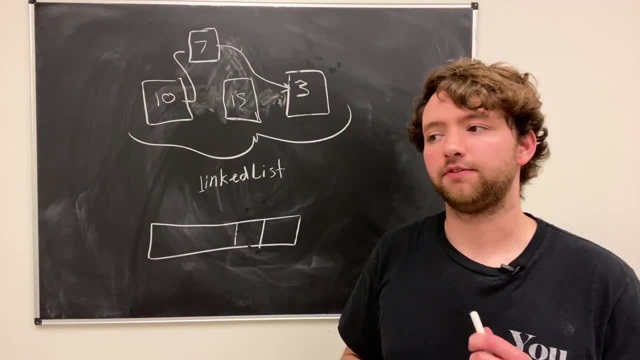 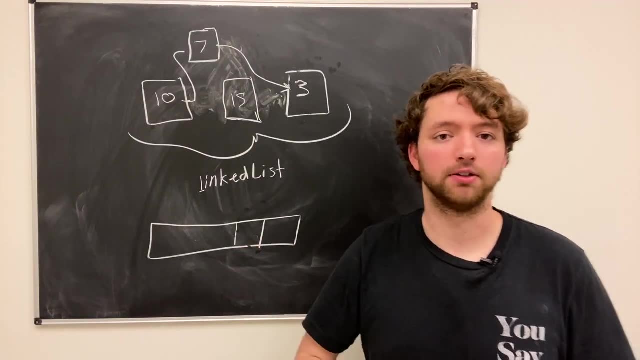 if you're in a data structures class or if you are doing something such as hash maps. Oftentimes if there's a collision, they'll use a linked list, So let me show you what that might look like. So let's say we have a table here and we want to insert data into this. 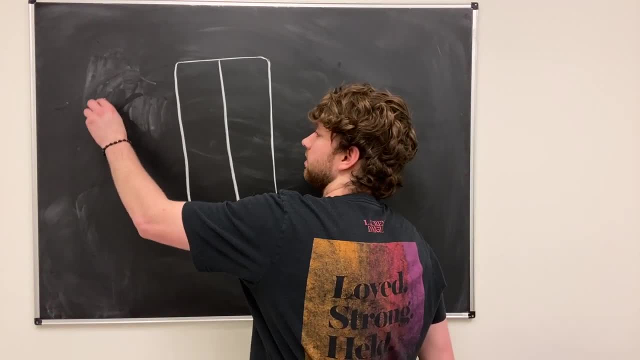 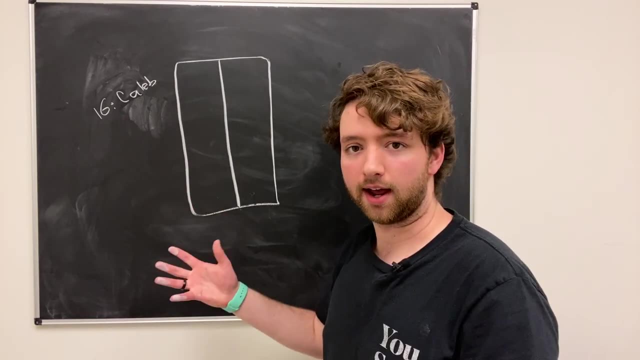 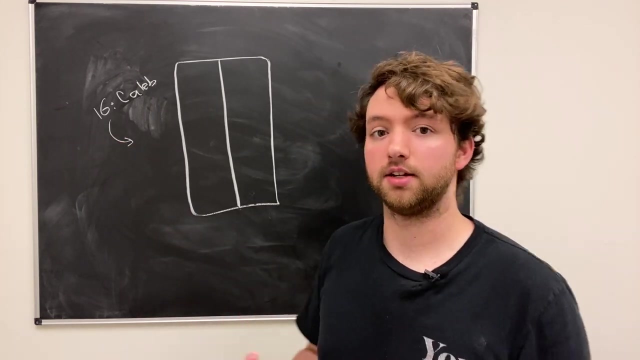 in a hash table like manner, We might have some data, such as 16 Caleb, where there's a key and a value. Well, this key is going to get hashed and I have videos on that process if you want. but basically it goes through some function to determine what the index is going to be And, let's say, it goes. 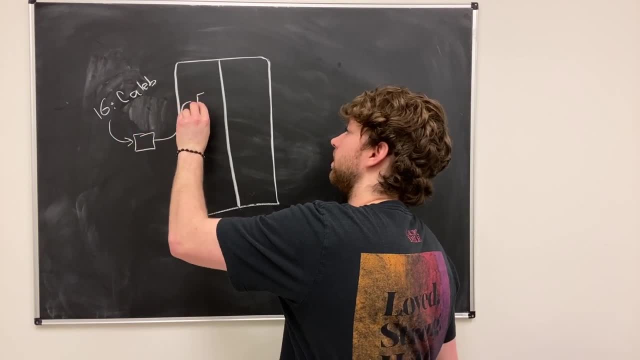 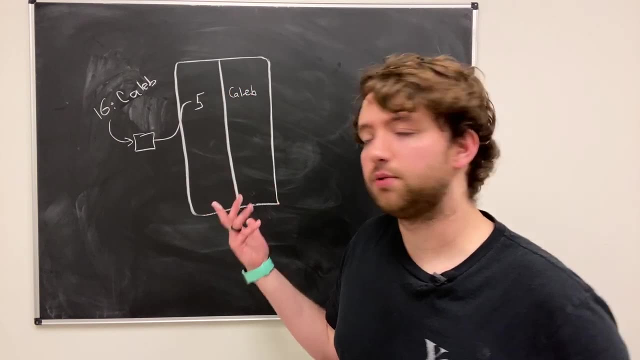 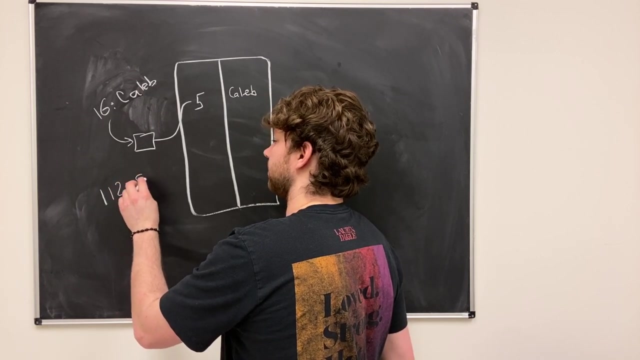 through that function and the final value is 5.. So it's going to go at index 5 and that's where Caleb goes. Well, let's say we do another one and this one. we have an association of like an id of 112, and this is Sarah.